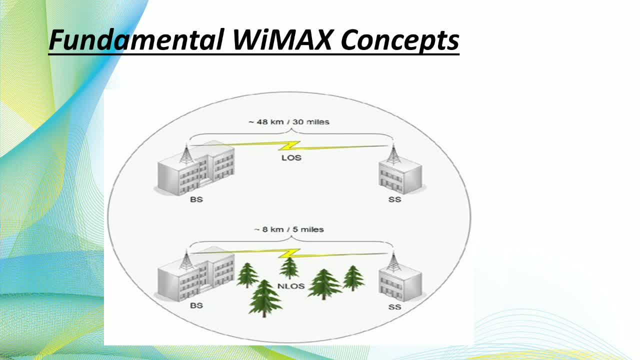 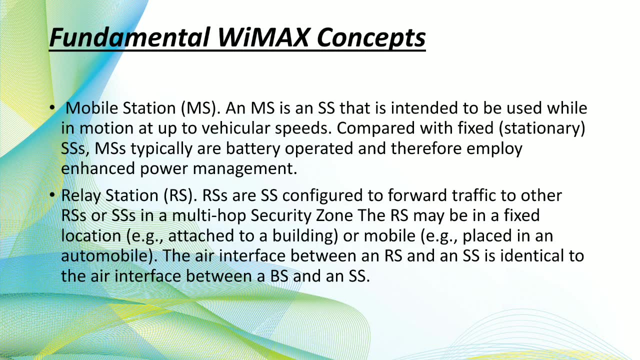 Now see Fundamental WiMAX Concept Diagrams. Now again see Fundamental WiMAX Concept Mobile Station MS. An MS is an access that is intended to be used while in motion at up to regular speed. Compared with fixed stationary SS and MS typically are battery operated and therefore employ enhanced power management. 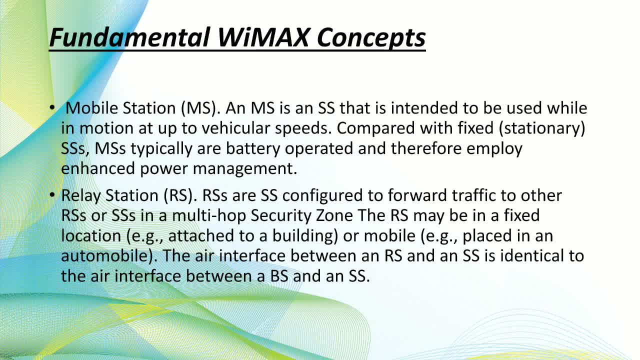 Relay Station RS. RSS are SS configured to forward traffic to other RS or SS. in multi-hole security zones, The RS may in a fixed location, eg attached to a building, or mobile, eg placed in an automobile. The Air Interface between RS and SS is identical. 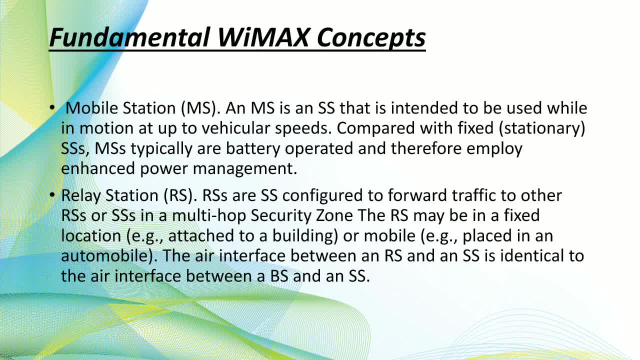 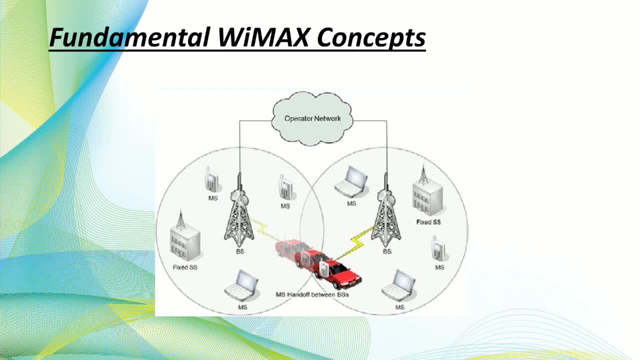 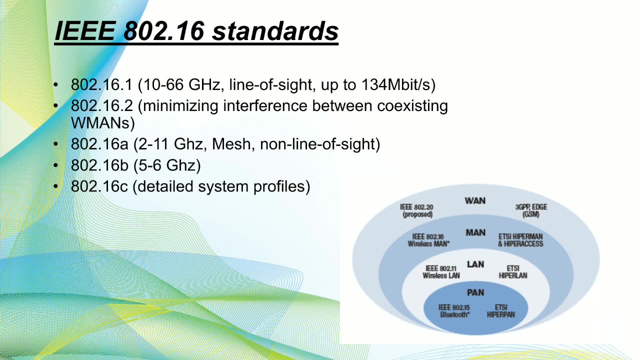 The SS is identical to the Air Interface between BS and SS. Again, see the Fundamental WiMAX Concept Diagram. Now move to the second topic: IEEE 802.16 Standard 802.16.1. 1066 GHz Line of Sight up to 134 MB per second. 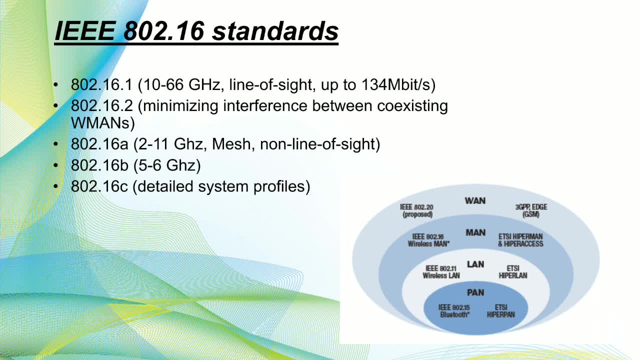 802.162- Minimizing Interference between coexisting WMANs. 802.168.2- 11 GHz- Mesh Line of Sight. 802.16b- 5.6 GHz. 802.6c- Detail System Profile. Types of WiMAX Connection. 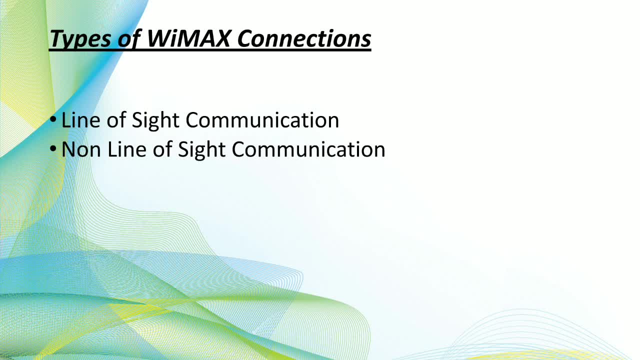 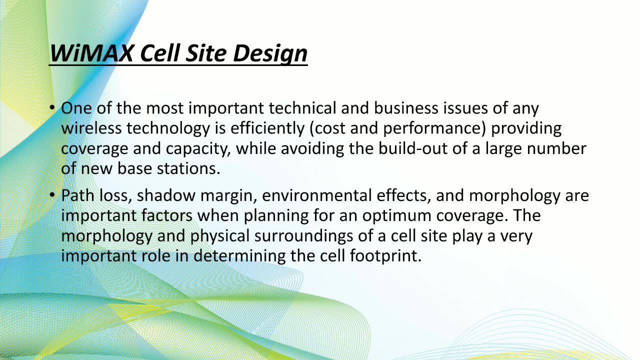 Line of Sight Communication. Non-Line of Sight Communication. WiMAX Cell-Sight Design. One of the most important technical and business issues of any wireless technology is efficiency, cost and performance, providing coverage and capacity while avoiding the build-out of a large number of new base stations. 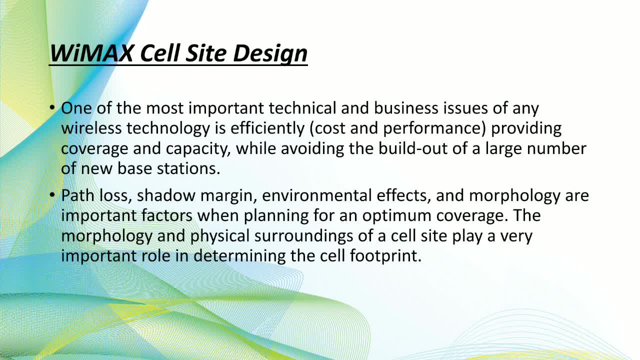 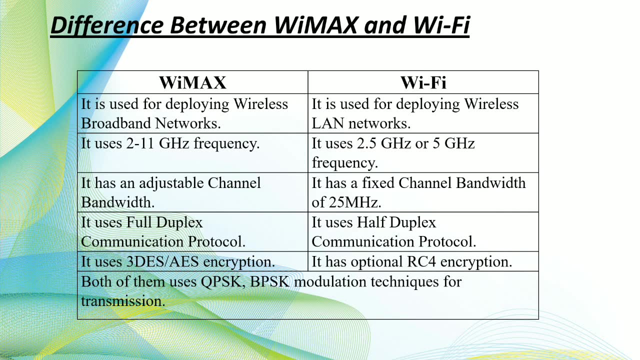 Path loss, shadow margin, environmental effects and morphology are important factors in planning for optimum coverage. The morphology and physical surroundings of a cell site play a very important role in determining the safety of a cell site. Difference between WiMAX and Wi-Fi: WIMAX: